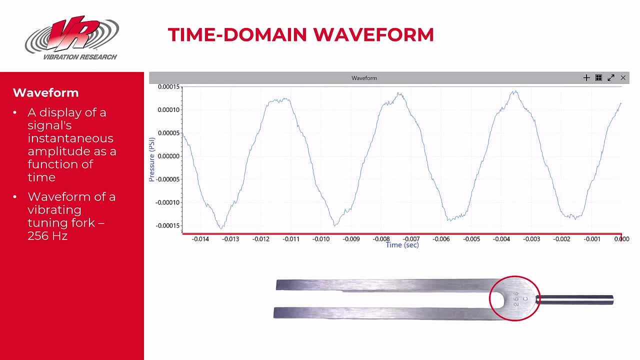 tuning fork. a tuning fork with a labeled frequency of 256 hertz. Note the simplicity of the waveform: It's close to a pure signed tone. When you examine the time domain waveform, you can tell that the time from one peak to another peak- one cycle- is about .004 seconds. 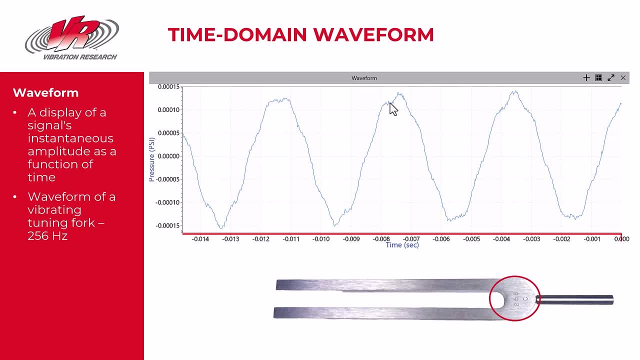 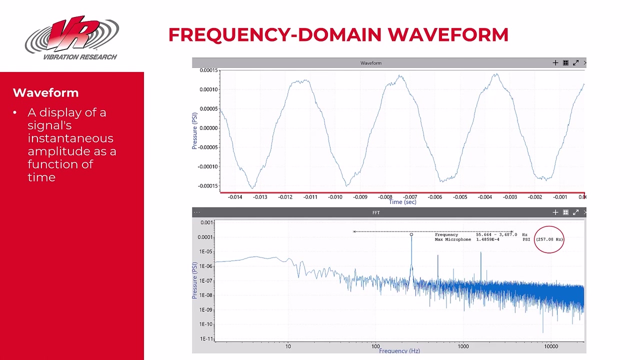 From, say, this peak to this peak, .004 seconds. roughly That would correspond to a frequency or inverses, a frequency of about 250 hertz, And that makes sense because the tuning fork is 256 hertz When the time domain waveform is transformed into the frequency domain. 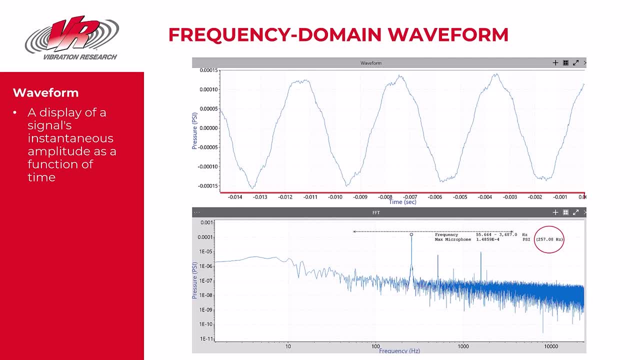 you can see that there is primarily frequency content at 257 hertz and some content at overtones above 257 hertz. This peak here this frequency is about .004 seconds. and this peak here this frequency is about .004 seconds. This peak here, this frequency is: 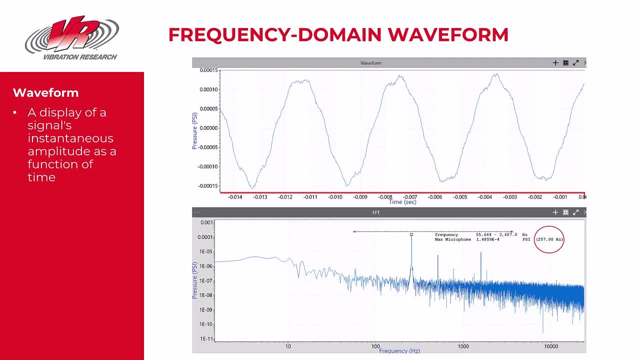 our main frequency, 257, 256, which is the tuning fork's value, and there is some overtones, But for the most part you see the frequency of that one tone. What this demonstrates is that a simple vibration, like a pure tone, from a tuning fork can be represented in 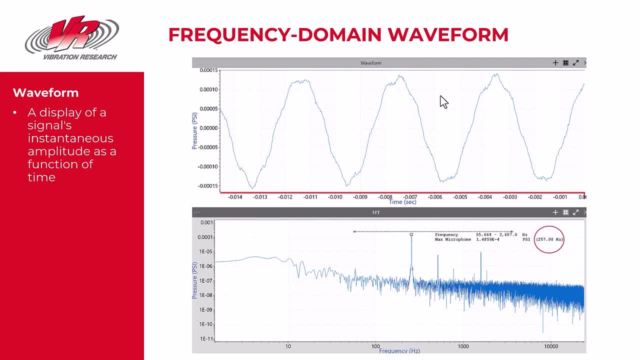 the time domain and it is even possible in that time domain to change the frequency. So it's a very simple concept. get a good idea of the frequency content by examining this waveform. However, the time domain waveform does not clearly indicate the harmonic content that is clearly visible. 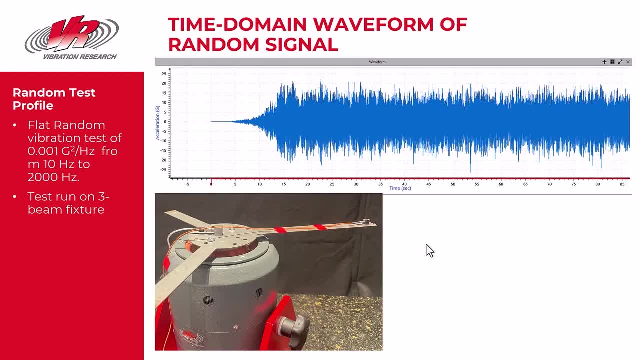 in the frequency domain. The second time domain waveform that I want to look at is from a random vibration test of that fixture. we've been working with the fixture with three arms, three beams, and note the complexity of this waveform compared to that of the tuning fork. It's very